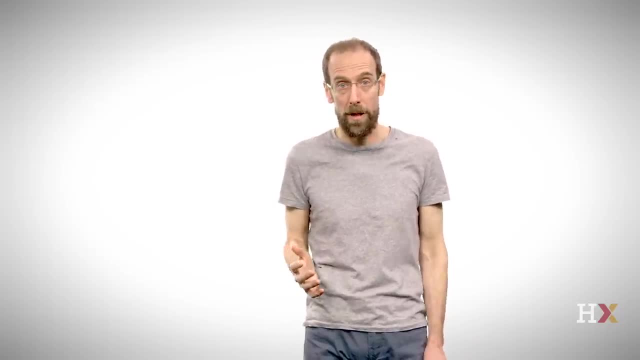 the problem is that cities differ in all sorts of ways that can affect health – other pollutants, employment, average age, etc. Epidemiologists do their best to separate out each of these factors and estimate the impact due to changes in PM alone. Here are results from one of the most influential air pollution epidemiological studies ever done. 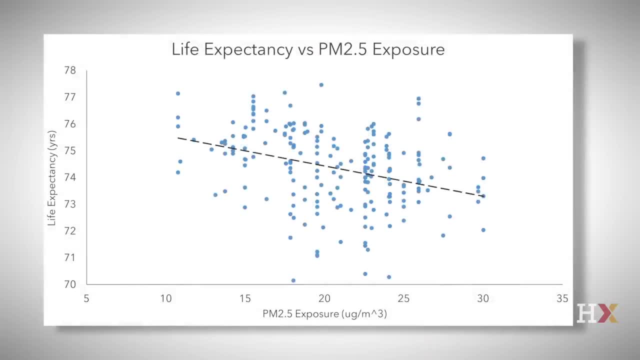 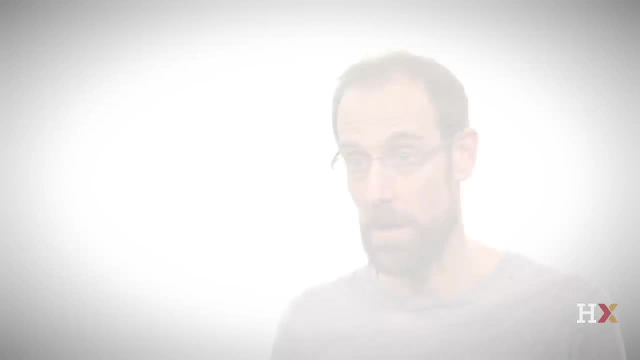 The net result is that an increase in PM2.5 of 10 micrograms per cubic meter decreases your life spine by roughly three-quarters of a year. The annual average PM2.5 values in Beijing approach 100. That means that residents' lives will be shortened by many years. Look up the PM levels. 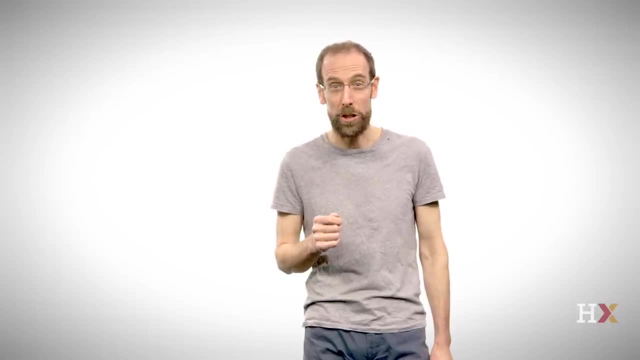 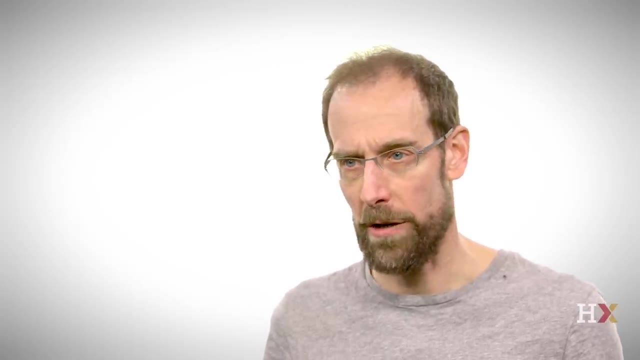 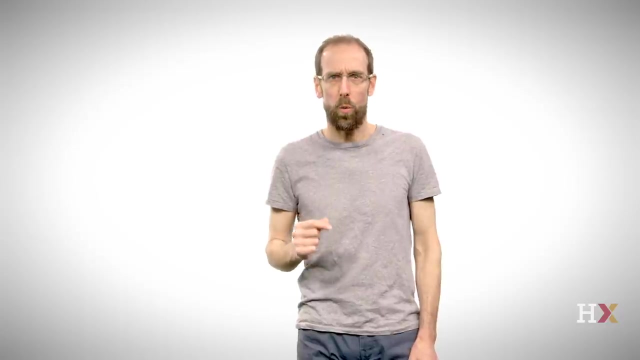 in the city you live in and figure out how much it is likely to shorten your life. How certain are these mortality estimates? My view is that the overall estimates are pretty accurate, though they still might easily have uncertainties of a factor of two or even more. However, it is much less clear which component of PM causes the problem. Some researchers think it's mostly due to metals and toxins, while others think that most of the damage is simply caused by the total amount of PM, which mostly comes from sulfates and nitrates. The answer really matters, as it should shape, where people put their efforts into pollution control. 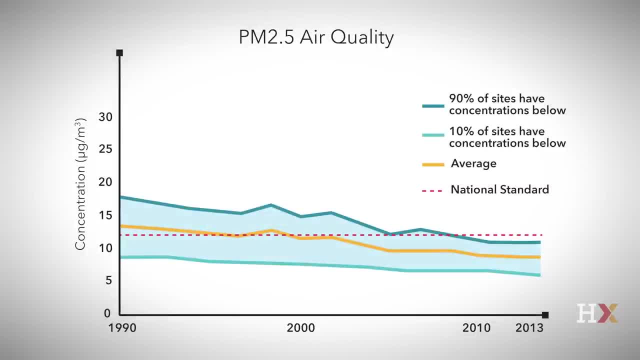 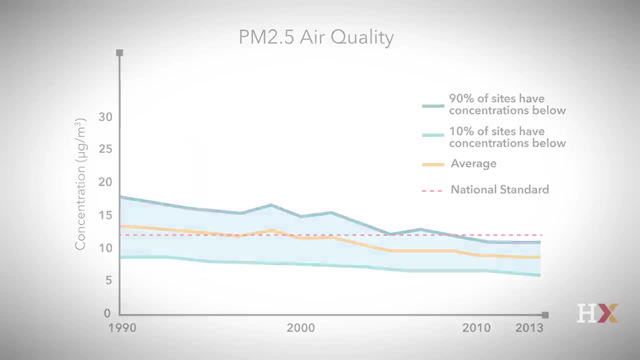 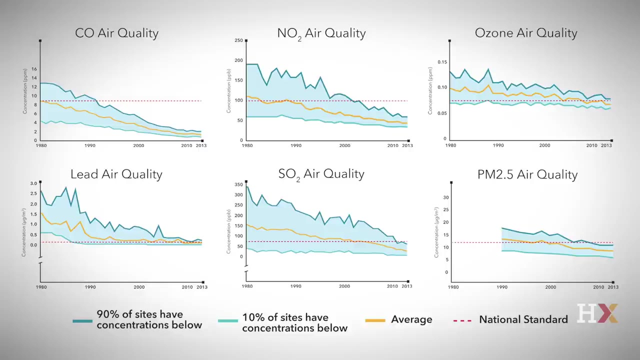 Average PM2.5 has fallen by about a third since the year 2000.. Now have a look at the time history of all six of the US criteria pollutants: Notice that progress for ozone and PM, the things that actually have the most health impact. 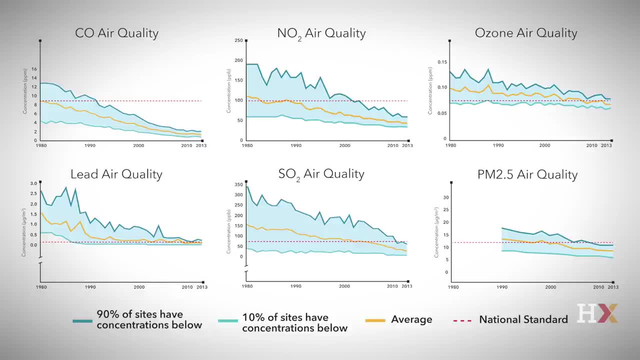 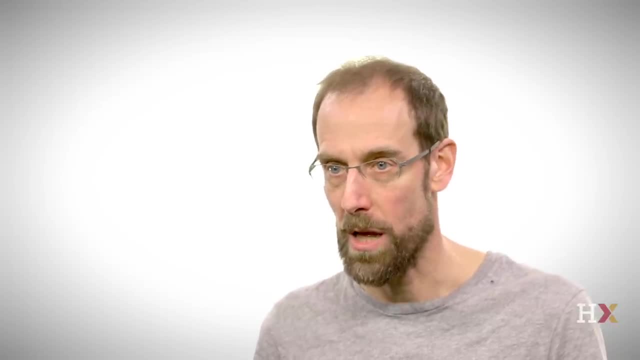 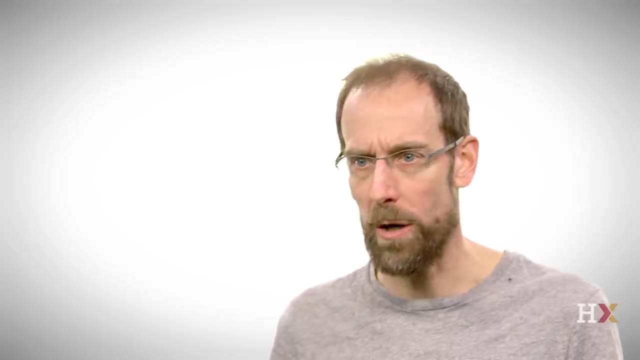 have been noticeably smaller than progress for the individual primary pollutants like lead or sulfur. I do not think this is chance. It's easier to control single pollutants than it is to control PM2.5.. and ozone, where many different sources, both natural and human, contribute in complicated 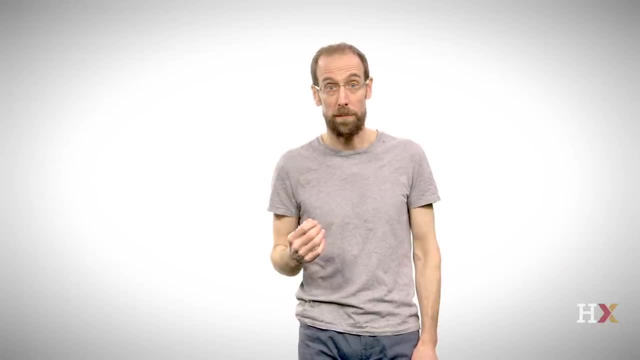 ways to the total pollution load. How have these reductions in pollution been achieved? In almost all cases, they have been achieved by technological changes in the way energy is produced or used, either by changing the process to reduce the production of the pollutant, as when lead is removed from gasoline, or by adding clean-up technologies like sulfur.